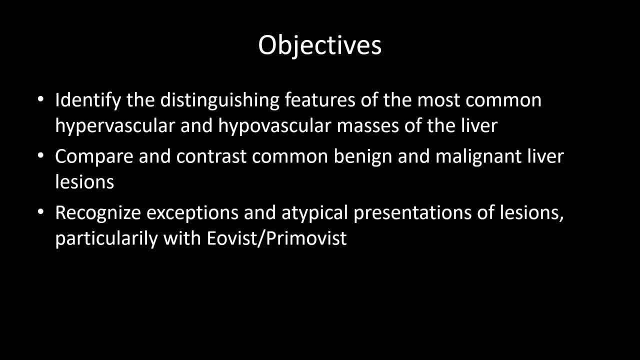 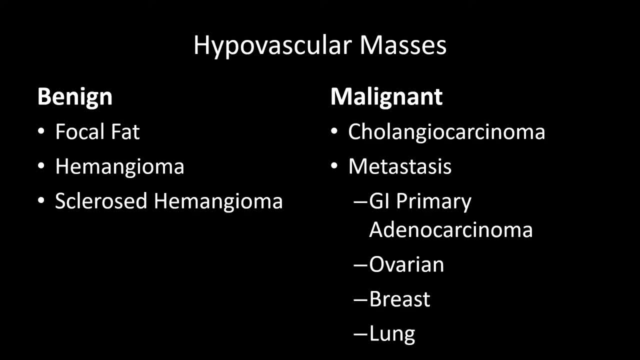 features, compare and contrast common benign and malignant masses and recognize some exceptions and atypical presentations. Let's talk about common hypovascular masses. In the benign category, I think of focal fat, which can be surprisingly mass-like and misleading, particularly on CT imaging, and you're 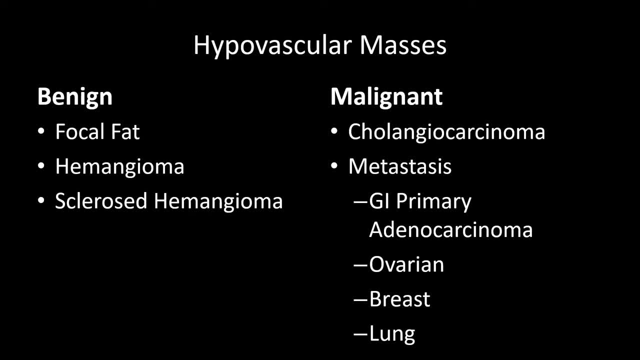 really going to lean on your in- and opposed phase MRI imaging to make the diagnosis of focal fat. Hemangioma in my mind is the most common type of mind, is the classic hypovascular mass. Some people may argue that it's hypervascular. It certainly 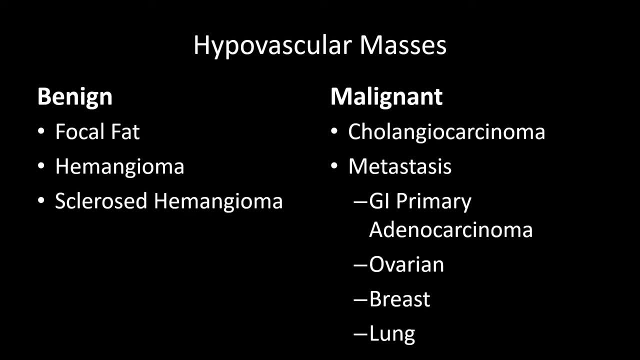 is a vascular mass, but its enhancement pattern to me is not as similar to the hypervascular masses we talked about in the first screencast as it is to some of these other hypovascular masses. Sclerosomangioma is a very challenging diagnosis. It is almost a diagnosis of exclusion. 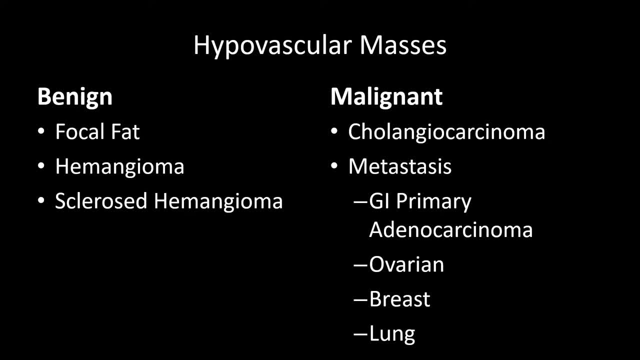 that should be made with biopsy, because its appearance is very similar to some of these malignant hypovascular masses. When I think about malignant hypovascular masses, the main primary malignancy within the liver would be cholangiocarcinoma and then the secondary. 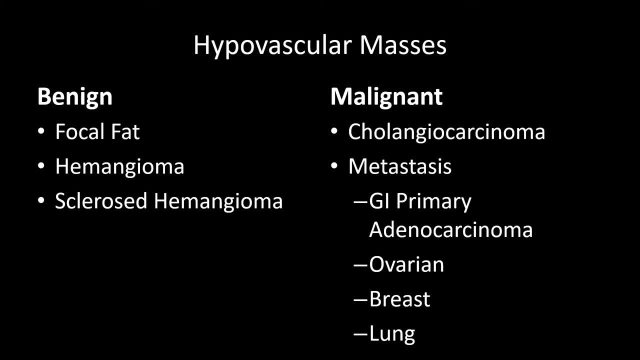 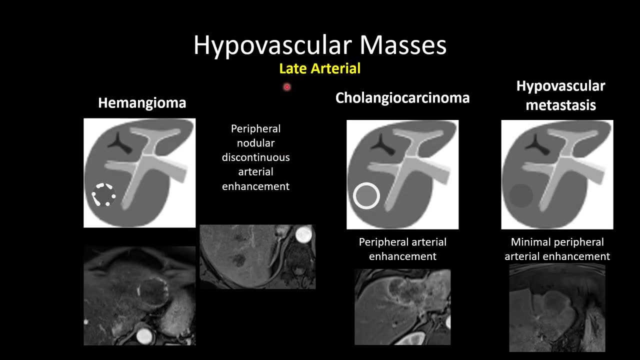 malignancies within the liver are going to be metastases And really adenocarcinoma. metastasis from any primary will have a similar appearance to cholangiocarcinoma within the liver. All right, so let's look at some of these enhancement patterns. Again, we're using a 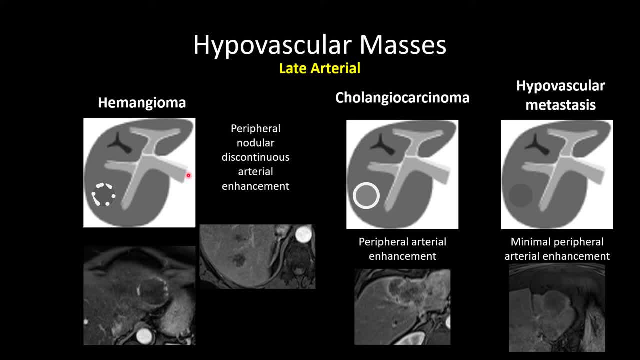 late arterial phase, where there is opacification of the hepatic artery and the portal vein but no opacification of the hepatic vein. In this late arterial phase, a hemangioma should show peripheral, nodular, discontinuous enhancement. Again, the enhancement must be discontinuous. There must be gaps. 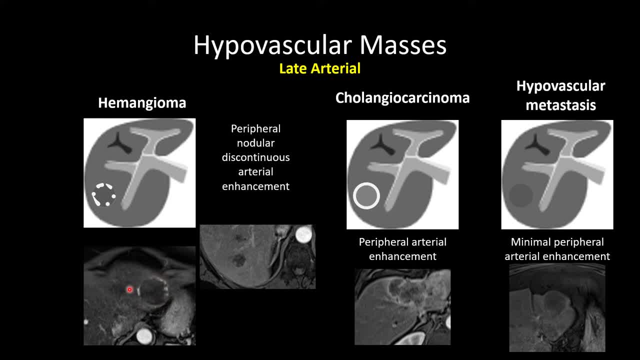 in the peripheral enhancement and that peripheral enhancement should appear nodular. Sometimes that nodule is very weak, or a single nodule as opposed to multiple nodules along the periphery. That distinguishes it from cholangiocarcinoma or hypovascular metastases, which tend to 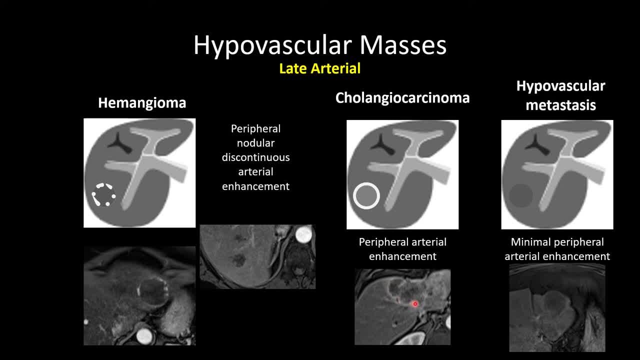 have a continuous, continuous peripheral enhancement. Sometimes that continuous, continuous peripheral enhancement can be somewhat nodular. It is often only on the periphery. but it should not be peripheral, nodular and discontinuous. Some hypovascular metastases, like this: GI primary adenocarcinoma- 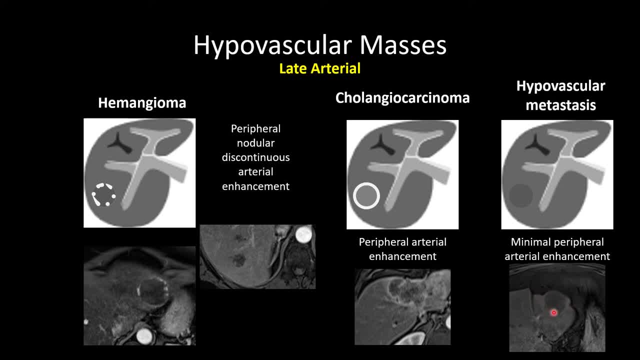 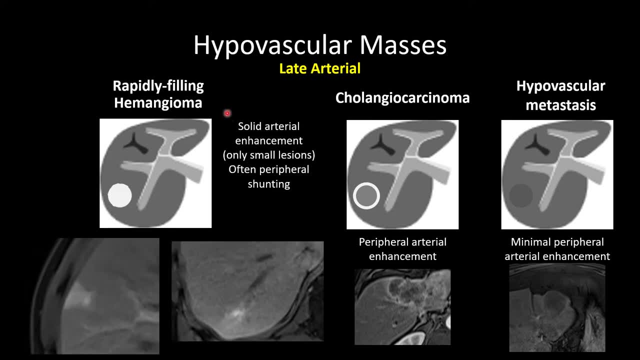 may show really minimal to no enhancement along the periphery in that early arterial phase. Remember that there are rapidly filling hemangiomas and these really fall back into a hypervascular differential and they may show solid arterial phase hyperenhancement. They tend to be less. 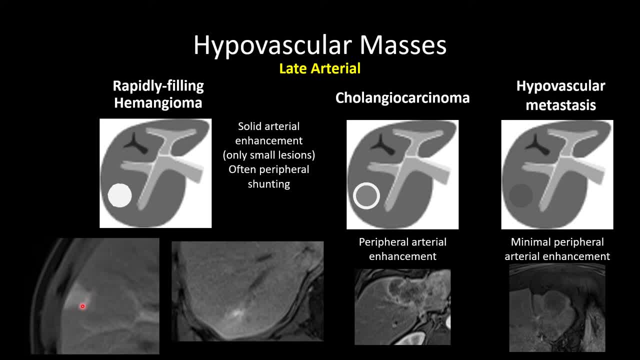 than two centimeters, even more commonly less than one centimeter, and are often associated with some degree of perilepsy. If we observe a benign hypovoidalázis, hypovan describing younger hormones as hyperphenogenesis, which is the taviterin overall. 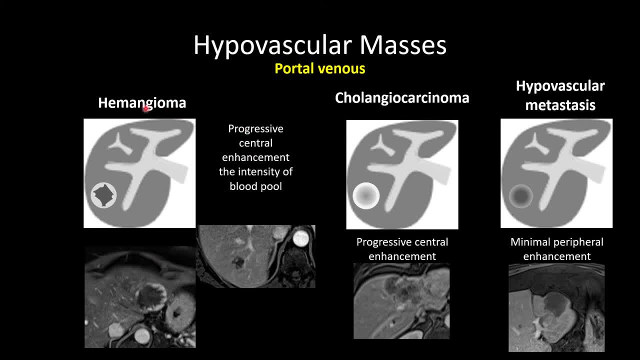 or the amylogenesis. increased platelet inhibition surge by hemangiomes at artificial neutrophils or in PGS, sigh perilesional shunting. They tend to again follow blood pool on subsequent phases of contrast. Now let's look at the portal venous phase. In the portal venous phase that haemangioma which showed that peripheral nodular discontinuous enhancement may start to show some degree of more continuous enhancement and the nondularity 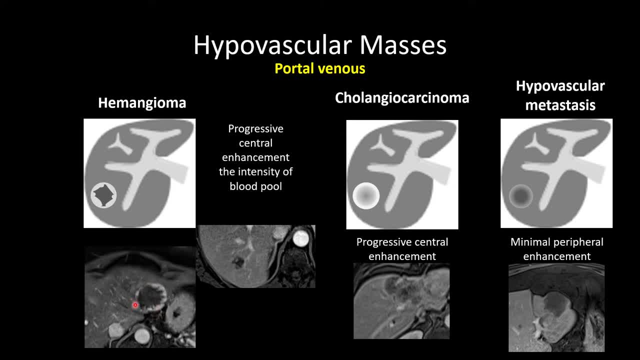 may be less apparent. However, it tends to remain peripheral, especially in that portal venous phase. In this much smaller hemangioma we can see another nodule. So again, we still have that kind of peripheral nodular enhancement And note that the enhancement should follow blood pool. 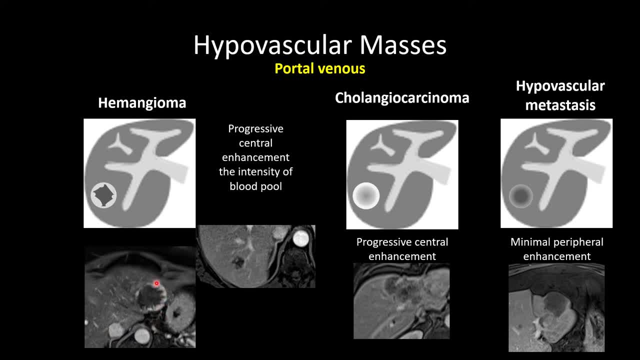 So we can see the IVC in the aorta here and we can see that the enhancement within that hemangioma by the enhancing portions of the hemangioma are very similar in signal intensity to the aorta and IVC. In terms of cholangiocarcinoma, we will also have progressive enhancement of the cholangiocarcinoma. 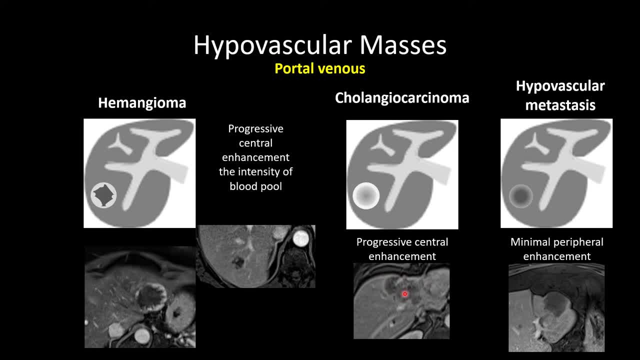 but that enhancement tends to not follow blood pool. Oftentimes in the portal venous phase that enhancement will be actually less than the aorta which we can partially see in this field of view, And hypovascular metastasis can have variable enhancement. Sometimes they will show. 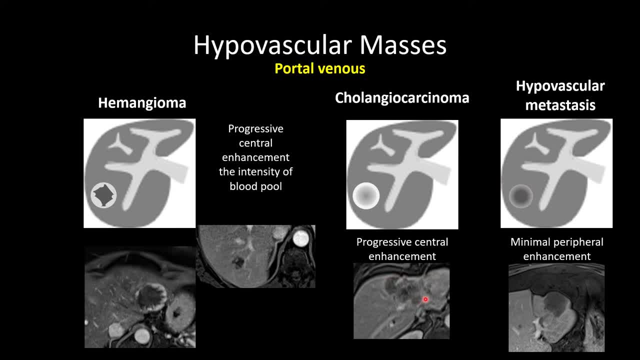 progressive enhancement. Sometimes they will show progressive enhancement. Sometimes they will show progressive central enhancement, similar to a cholangiocarcinoma. Other times they will show little to no enhancement. Also note in this large intrahepatic cholangiocarcinoma. 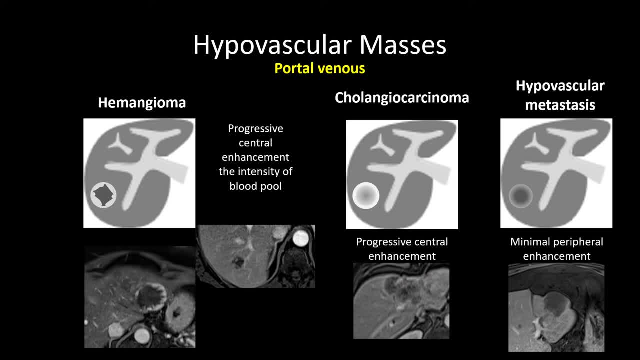 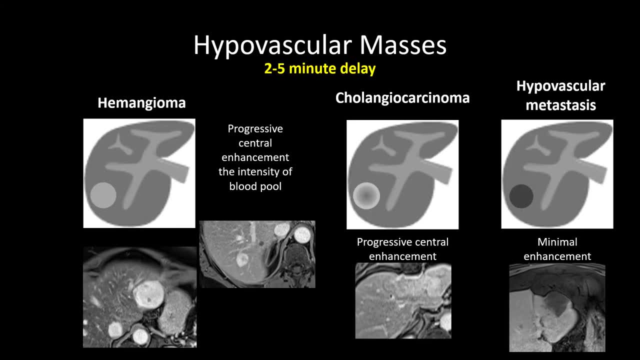 we do see some capsular attraction, another classic feature for intrahepatic cholangiocarcinoma. As we move out to the two to five minute delay, you're going to see continued progressive central enhancement within the hemangioma. Okay, so now this hemangioma is homogeneously enhancing. 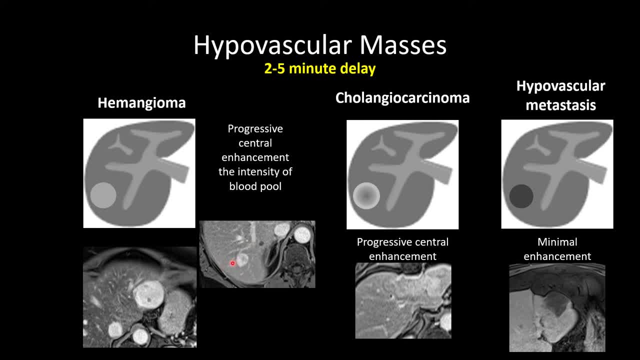 or near homogeneously enhancing, as is this smaller one. Note when you compare the hemangioma to the aorta and IVC, it is very similar in signal intensity to the blood pool. Same with this hemangioma, which is very similar in signal intensity to the blood pool. When we look at this, 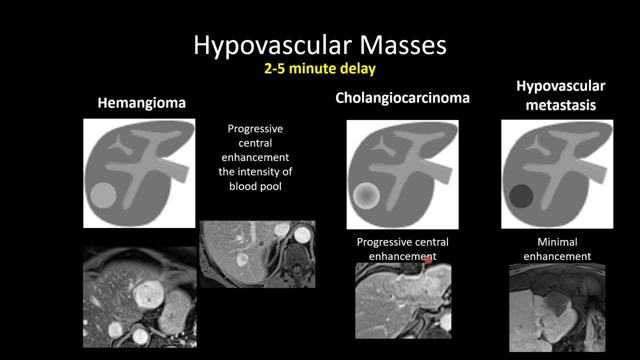 cholangiocarcinoma, intrahepatic cholangiocarcinoma- we see that there is progressive central enhancement. There's near homogenous enhancement now of the mass, but that enhancement is actually less than blood pool. The progressive central enhancement within the 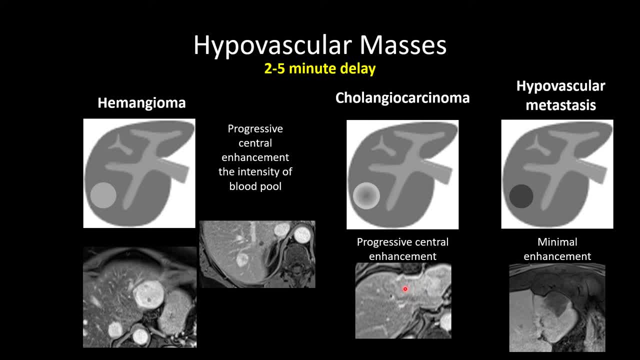 cholangiocarcinoma is somewhat due to the fibrotic nature of the tumor. and third, spacing of gadolinium into hypovascular regions of tumor. that allows the gadolinium to accumulate over time. In this delay, we see, maybe, some minimal performance. We see some minimal performance. We see some minimal performance. 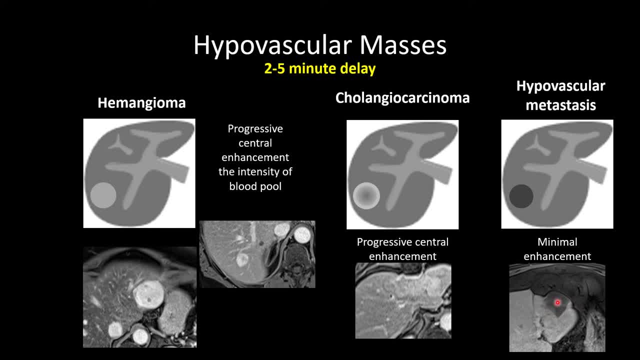 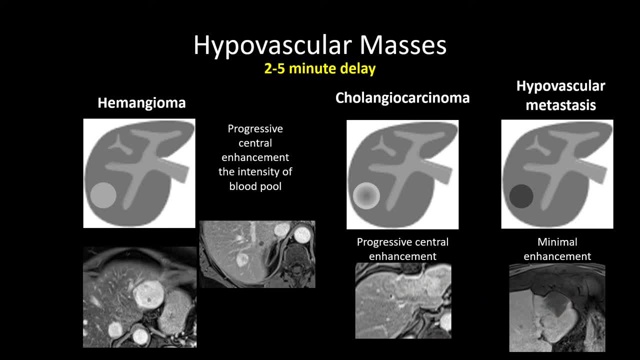 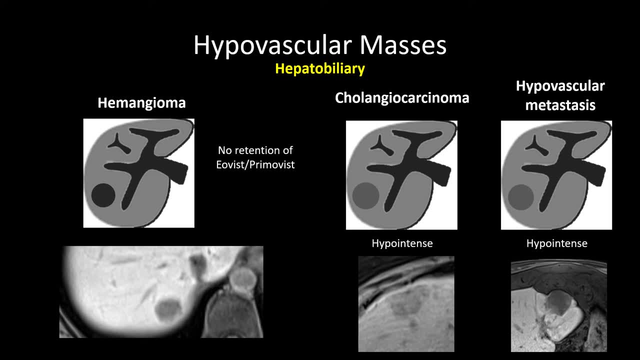 metastasis, but it could look very similar, if not identical, to the cholangiocarcinoma. When we move to the hepatobiliary phase, we should see uniformly across almost all hypovascular masses, whether they're benign or malignant, hypointensity on the hepatobiliary. 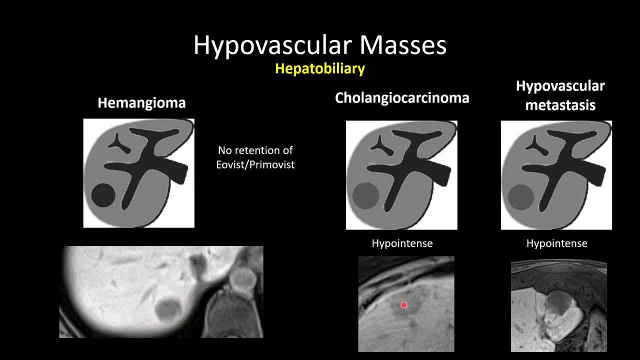 phase. So hemangiomas are hypointense, cholangiocarcinomas are hypointense and metastatic lesions should be hypointense If it is isointense. on the hepatobiliary phase one, make sure the blood pool is cleared, So make sure there is no contrast remaining in the aorta. 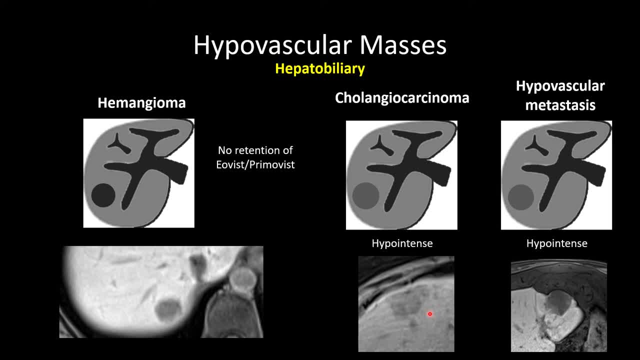 or IVC. And then if there is still hypo or isoenhancement or uptake of eovist, there are some malignant lesions that can retain eovist in addition to FNH. So you're going to have to dig a little bit deeper into the signal intensity and imaging features of the mass. 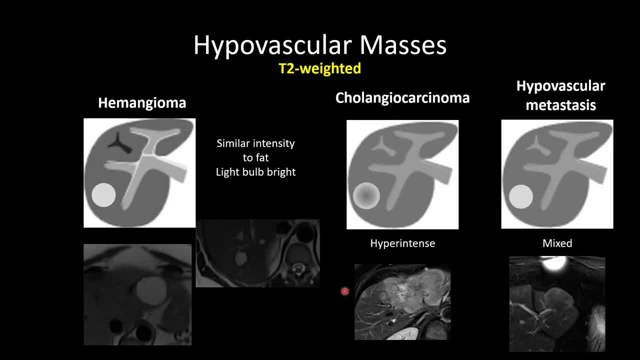 On two-weighted imaging we're going to see that a hemangio hemangioma is moderately to markedly hyperintense. Now it is not as hyperintense as fluid, So the gallbladder or the CSF within the spinal cord tend to be slightly hyperintense to a hemangioma. 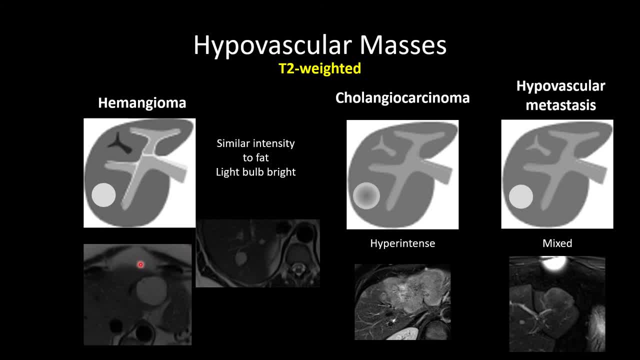 but the hemangioma actually will have similar signal intensity to fat. So if you look at the mesenteric fat or the subcutaneous fat, hemangiomas are typically isointense to that subcutaneous or mesenteric fat And you can see, that's the. 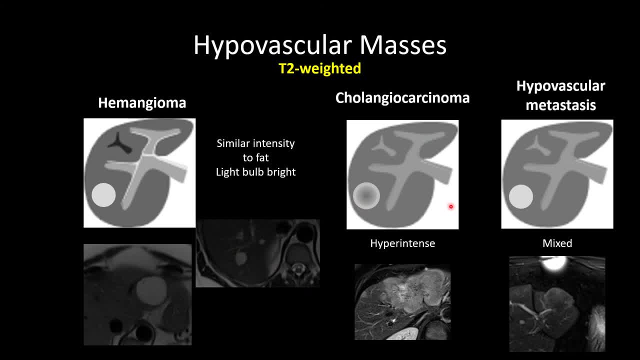 case with both of these hemangioma. In terms of cholangiocarcinoma, it does tend to be hyper intense. I would say that the hyperintensity is mild to marked. So, as opposed to the hemangioma, which is moderate to marked, this is mild to moderate. Okay, Not very rarely does the 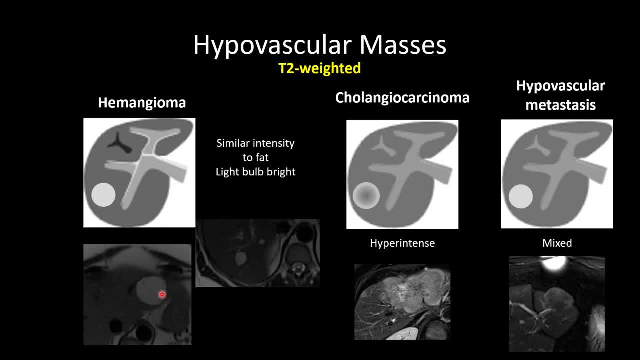 hyperintensity, get to the mesenteric fat. So if you look at the hemangioma, it does tend to be to the degree that a hemangioma is, although I have seen some that are quite hyper intense. Hypovascular metastases are highly variable. They tend to be mixed in terms of their hyperintensity. 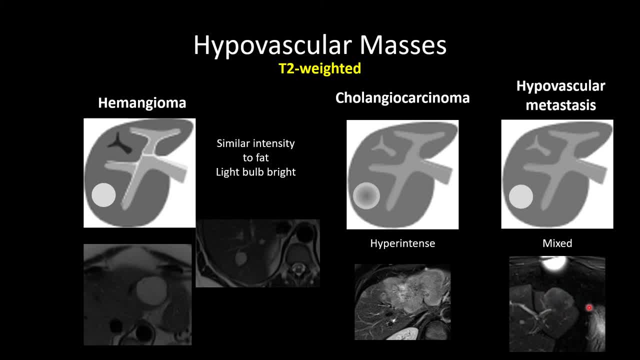 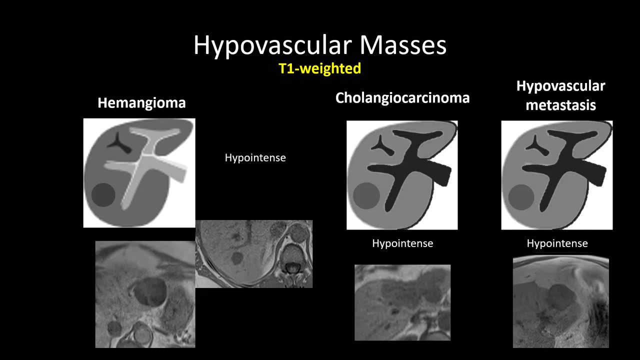 on T2-weighted imaging, Oftentimes they're mildly hyper intense relative to the liver, unless you're talking about some sort of mucinous type of metastasis which can then mimic fluid On T1-weighted imaging, similar to what we talked about on our hypervascular metastases, or 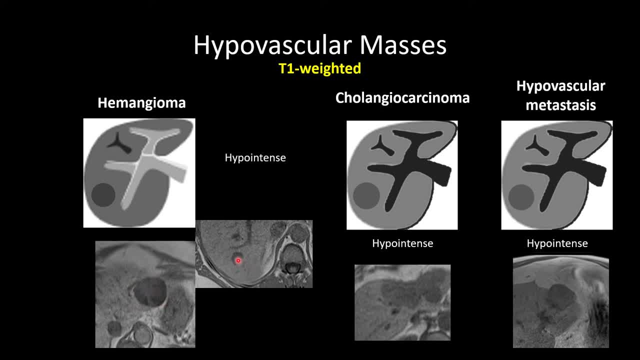 hypervascular masses screencast. real nodules and masses tend to be T1, hypo-intense. Okay So hemangioma, cholangiocarcinoma, adenocarcinoma, metastasis- Real masses in the liver tend to be: 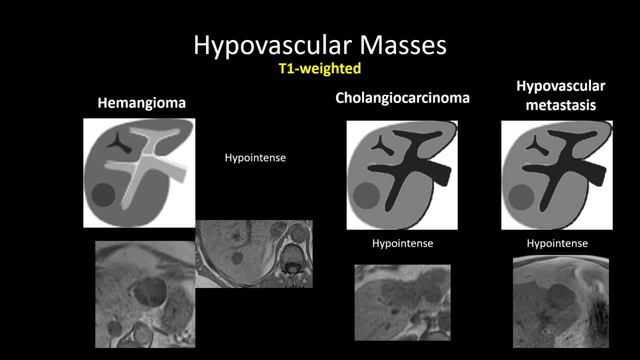 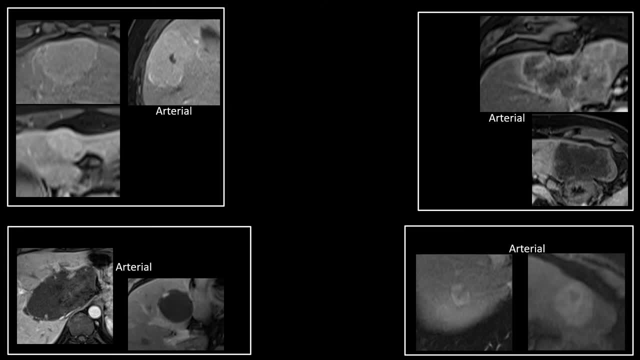 hypo-intense, to the background liver. All right, So let's just review some of the masses that we've seen in the first two screencasts. These are some different examples of hypo- and hypervascular masses. Look at this arterial phase. Look at the four different boxes. They each contain a different mass that we've covered so far. 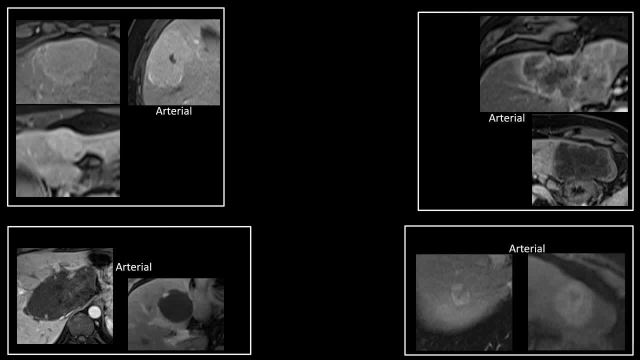 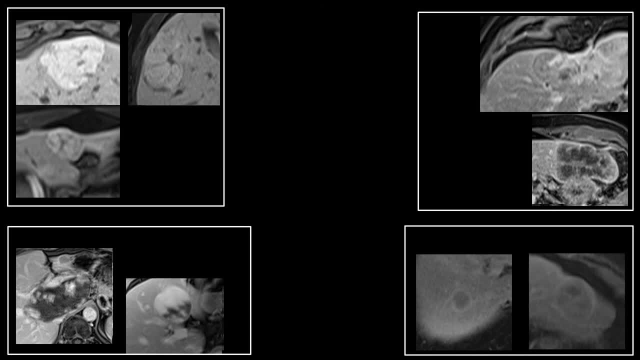 And try and think, just based on the arterial phase, which box you think contains which mass or nodule. Now we're moving to a more delayed phase. Here we can see this mass, which was hypervascular, is equilibrating, This mass which showed peripheral 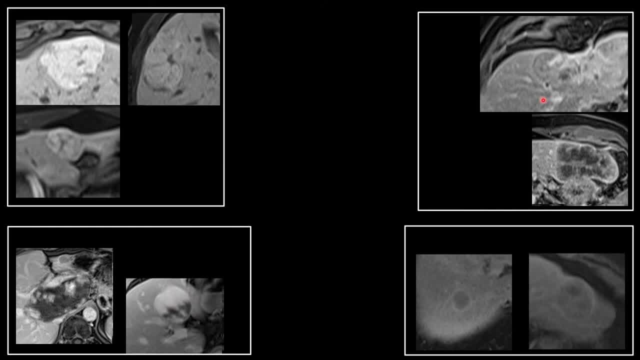 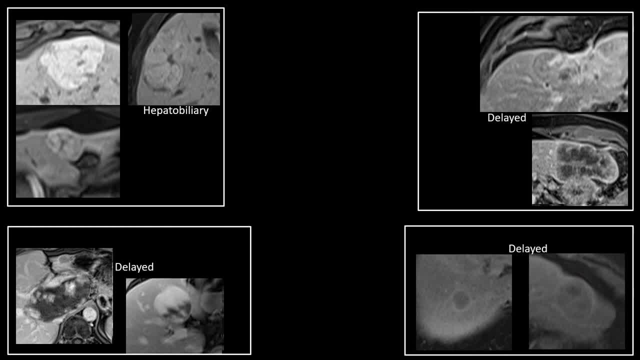 And here we see washout and capsule appearing. So if we have hepatobiliary phase and delayed phase, we can say that this is an FNH, This is a cholangiocarcinoma, although again, adenocarcinoma, metastasis could have a similar. 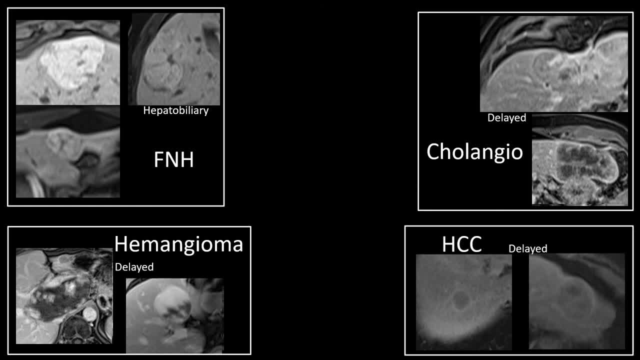 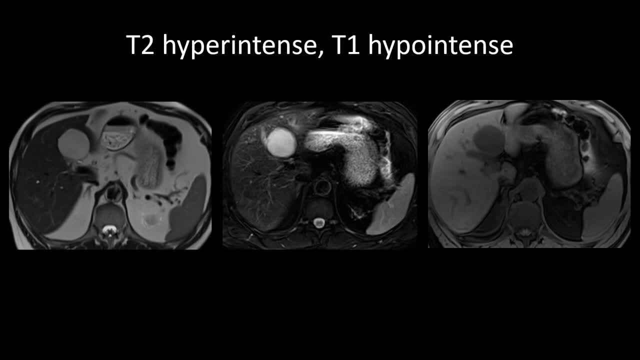 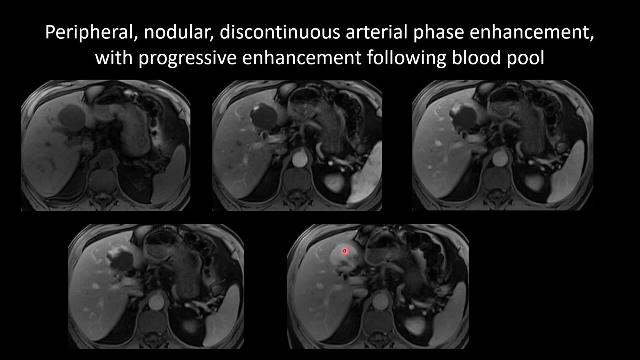 appearance: Hemangioma and hepatocellular carcinoma. Let's look at a couple more examples Again. classic example here: T2- hyper-intense, T1- hypo-intense. Notice the signal intensity is very similar to that. We have peripheral nodular discontinuous enhancement, progressive enhancement. 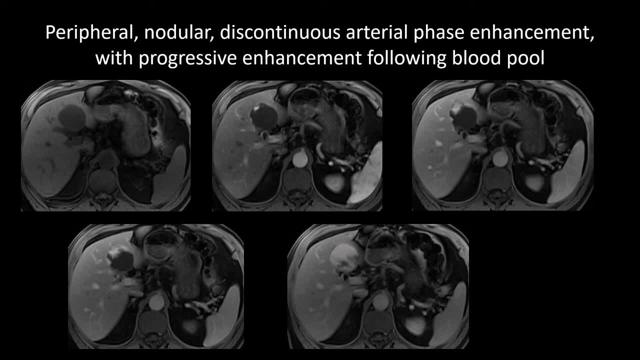 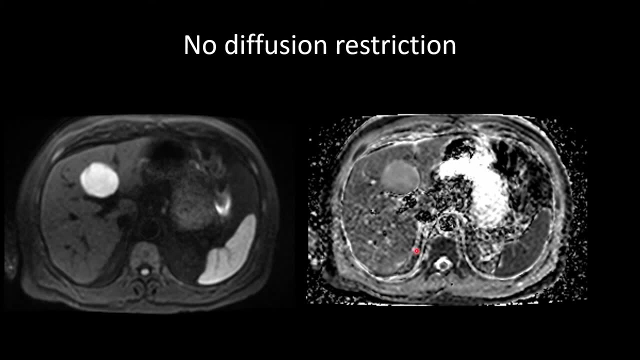 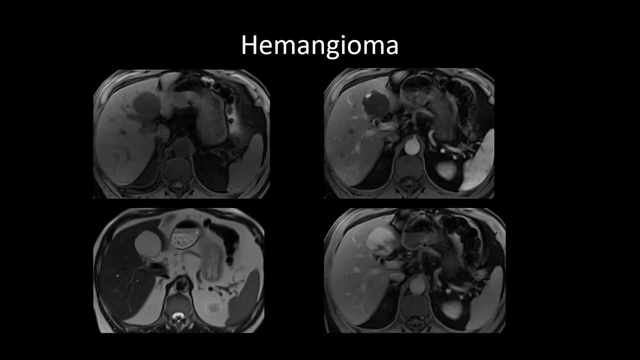 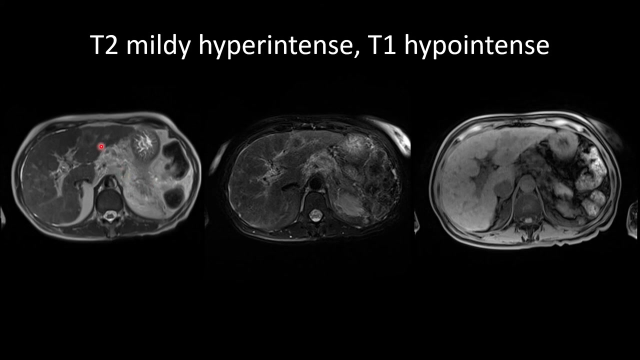 nicely following the blood pool. There's not really diffusion restriction here. It's mostly T2 shine-through with the mass being hyper-intense to the background liver on our ADC map And this is a classic hemangioma. Here we have another mass a little more challenging. We see this rim of T2 hyper-intensity. 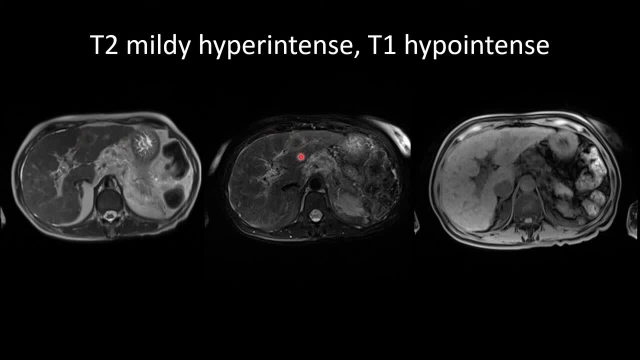 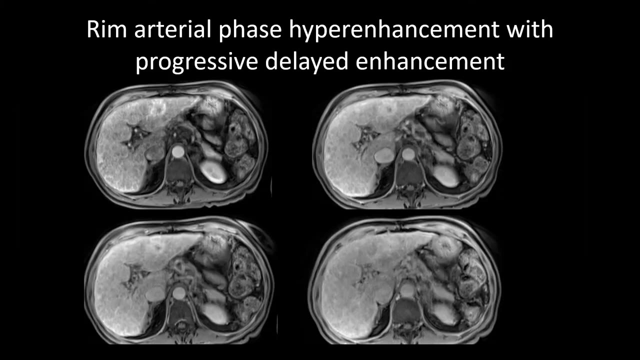 that may be slightly more apparent on our fat-saturated image and see some central hypo-intensity. On our pre-contrast T1 weighted gradient, recalled echo, we see it is hypo-intense to the background. liver: On our contrast enhanced imaging we have rim arterial phase hyper-enhancement. Notice this liver is very 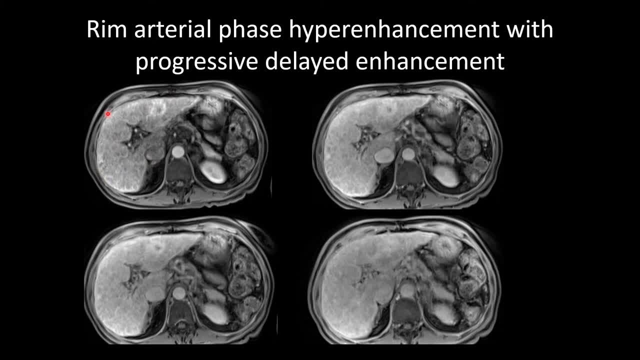 heterogeneous. so this is a person with cirrhosis And so we might be thinking hepatocellular carcinoma. but in this case that rim arterial phase hyper-enhancement is not going to be consistent with hepatocellular carcinoma, or at least a typical hepatocellular carcinoma. 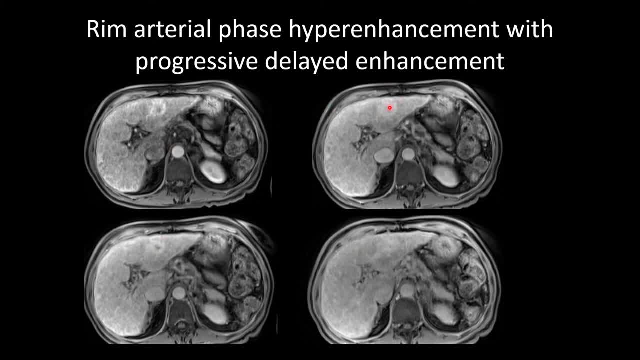 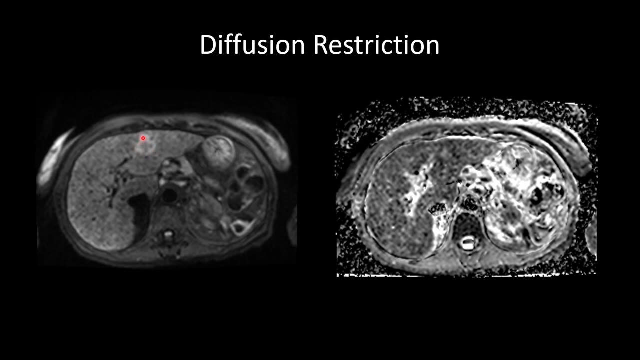 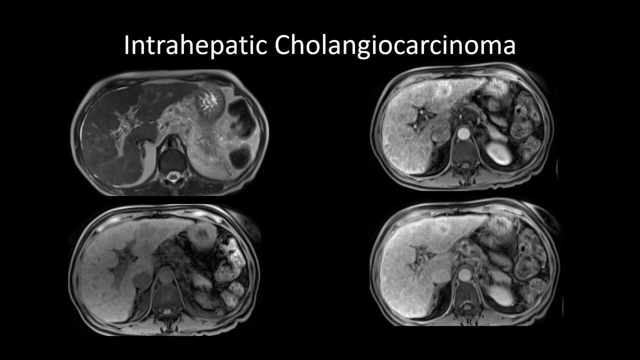 As we progress through our phases of contrast, we see progressive enhancement, but that progressive enhancement is slightly less than blood pool. This mass does show some diffusion restriction, particularly along the rim of the mass, And this is consistent with an intrahepatic cholangiocarcinoma. 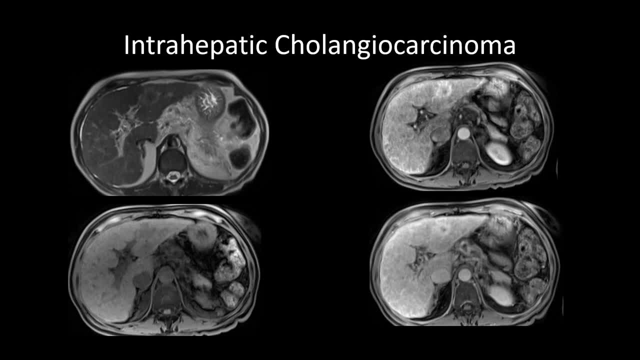 Again this same enhancement pattern you could see with a breast cancer metastasis, an adenocarcinoma of the lung, metastatic to the liver or a GI primary, But this turned out to be an intrahepatic cholangiocarcinoma. 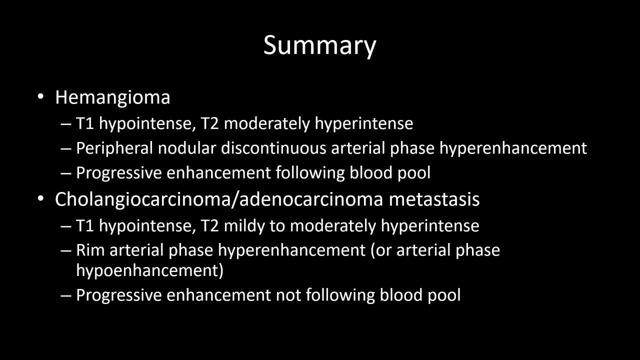 In summary, hemangiomas: T1 hypo-intense, moderately to markedly T2 hyper-intense, and it really is similar to that subcutaneous fat. It has to have peripheral nodular, discontinuous arterial phase hyper-enhancement If it's contiguous or not peripheral or not nodular. 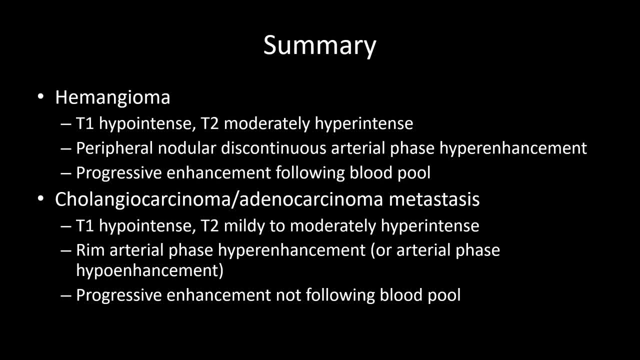 then you have to say it's an indeterminate nodular mass. The progressive enhancement should follow blood pool And realize that a sclerosed hemangioma is not going to follow this pattern but is going to more closely mimic the pattern that we described with cholangiocarcinoma or adenocarcinoma metastasis.